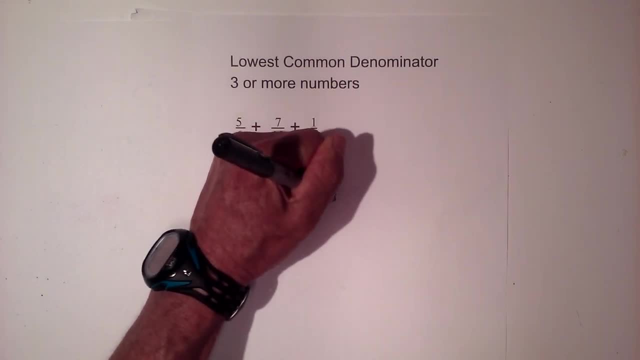 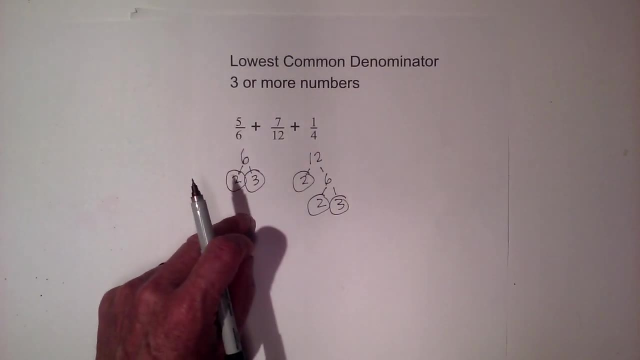 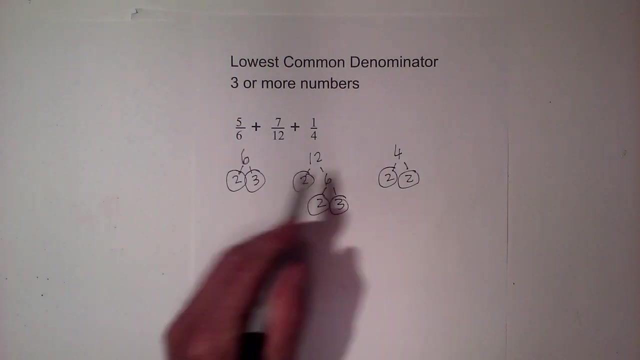 times 6 and then 2 times 3. and the reason why i like a factor tree is because really, if you know the multiples of 2 and 3, you really can do a factor tree pretty quickly on just about any numbers. okay, and then 2 times 2 is 4, so i've circled all the prime numbers. so that's step one create. 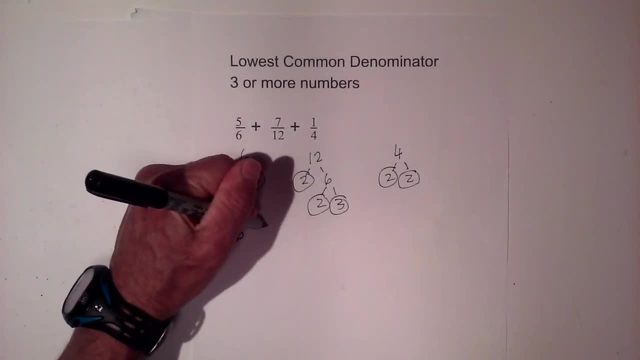 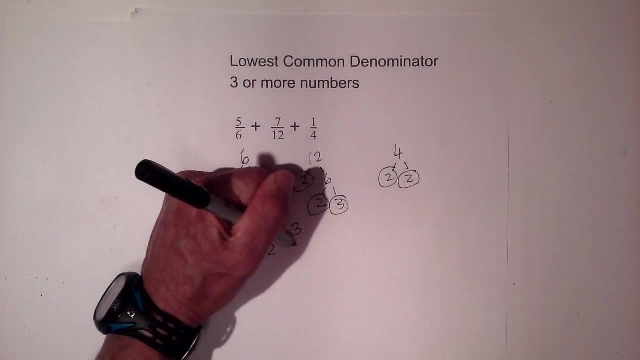 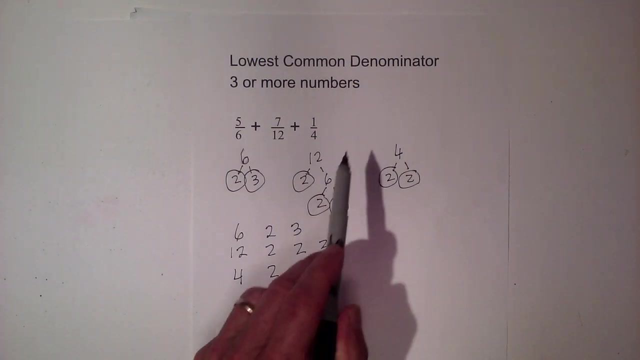 a factor tree. next, i'm going to write each number down and this step just helps cut down errors. you do not have to complete this step, but it really will prevent errors. and i'm just writing down the prime numbers and now all we need to do to get the lowest common denominator. 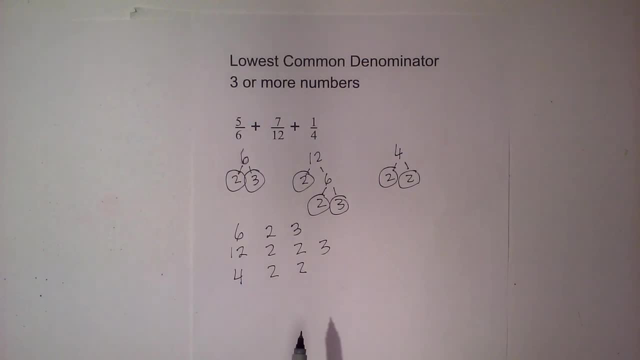 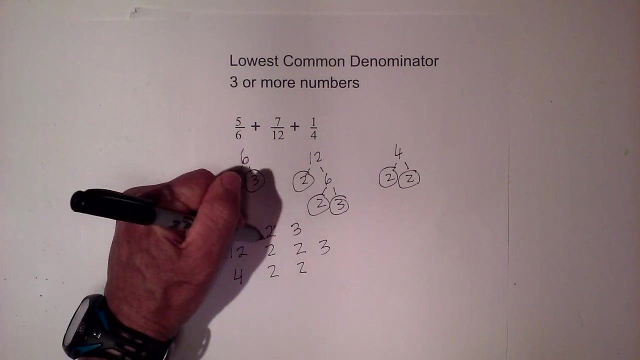 is: multiply all these prime numbers together. however, there is one rule you need to follow: if the number is in more than one of these numbers- the original numbers- then you only use it once. and here's what i mean: 2 appears in 6, 12 and 4, so i'm going to cross each of these out. 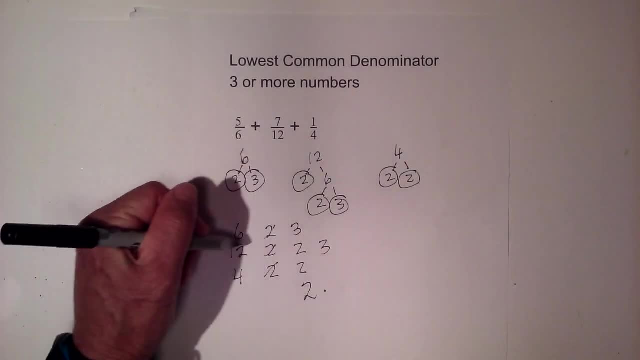 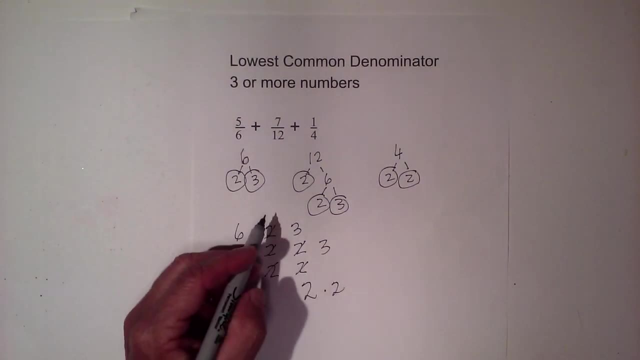 and only multiply it once again. we have a 2 and it's in two of the numbers, so i'm only going to use it once. and then we have a 3 in 6 and 12, so i'm only going to use it once. so now i have all the 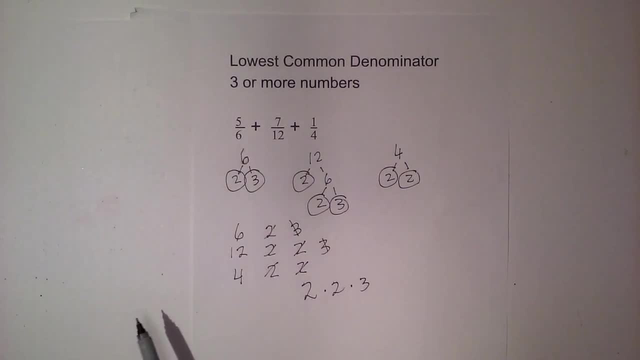 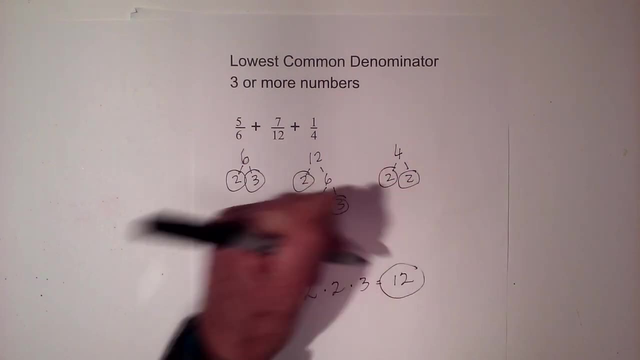 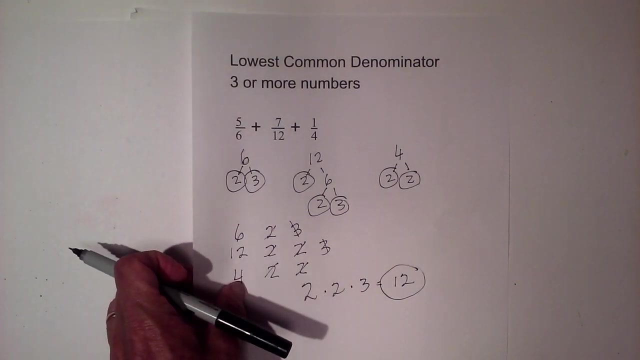 numbers crossed out and i'm going to multiply these prime numbers together: 2 times 2 is 4, and 4 times 3 is 12.. okay, so 12 is the lowest common denominator and that one is a very basic one. i will get a little more challenging problems as i move on. so now let's try what if we have this? 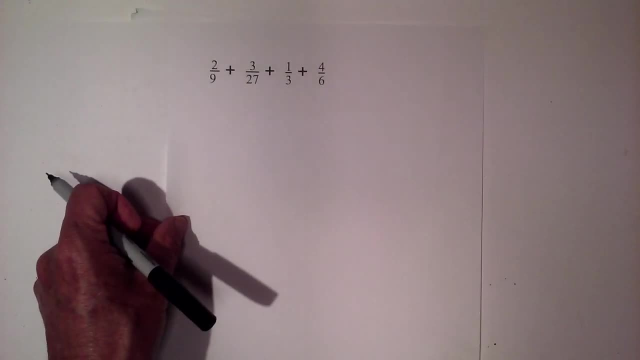 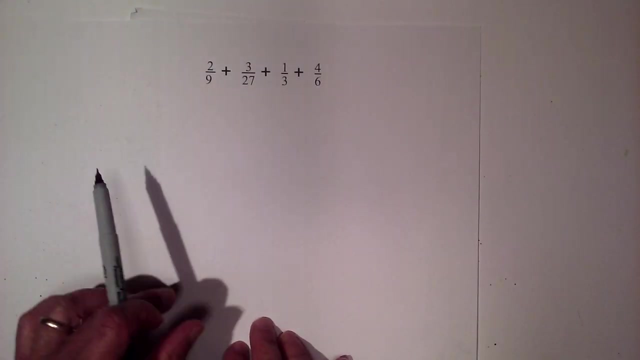 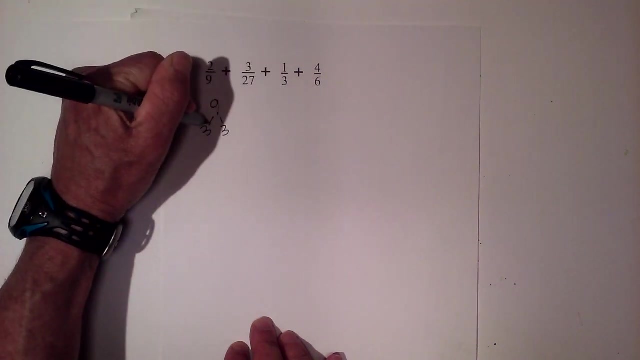 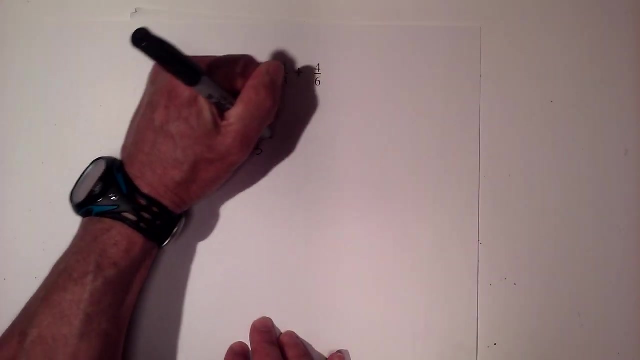 what if we have four numbers? okay, and by trial and error, it's challenging find the lowest common denominators of four numbers. uh, and so let's get started. let's create factor trees. three times three is nine, circle the primes and then 27, and with 27 i have three. 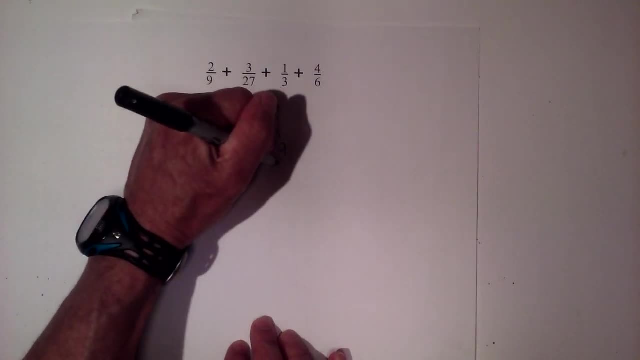 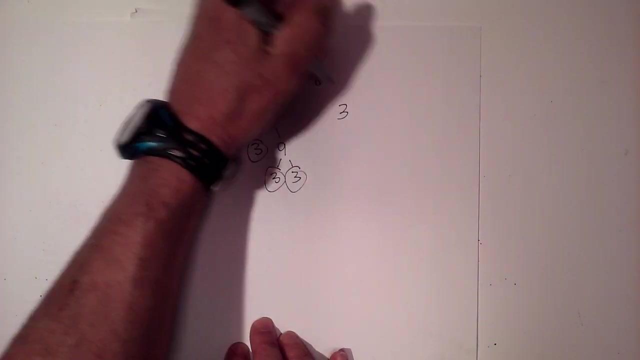 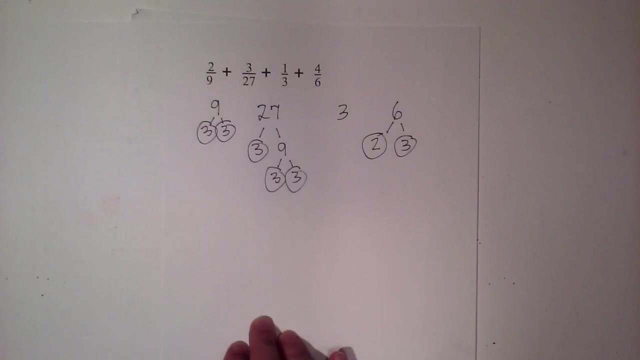 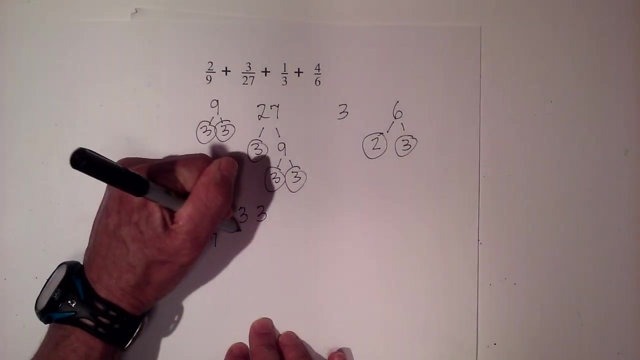 times nine, circle the three because it is prime, and then three times three, and then obviously three is already prime. and then 6 is just two times three. circle the two and three because it is prime. now i'm going to write down all of my prime numbers. okay, seven is three times three times three, and then obviously 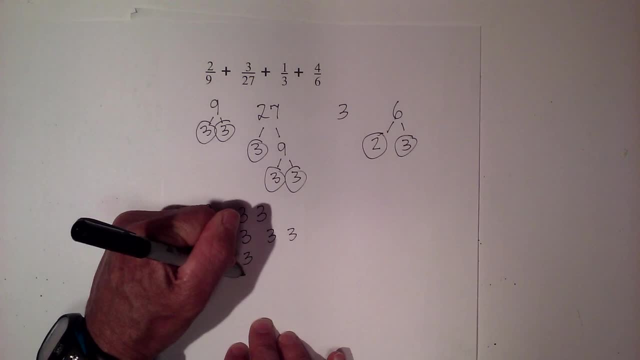 three, and i'm gonna go ahead and write the three here and then six is two times three. so now i follow my rules again. if the three, if the number is found in more than one number, then i'll only use it once and basically i'm multiplying all the prime numbers together. 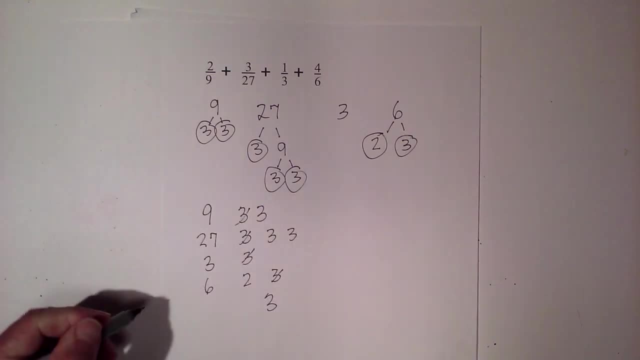 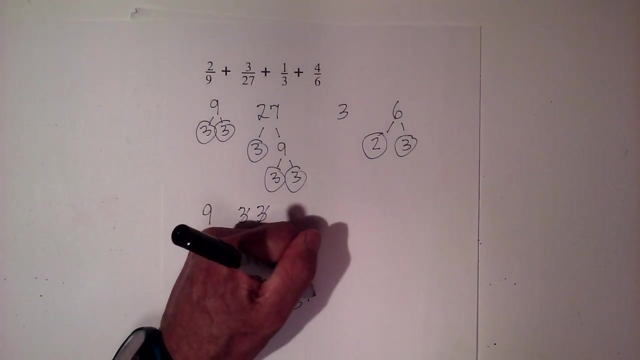 so this three is found in three of the numbers. and then we have this: three is in two of the numbers. this, there's three, it's the same three. so there's another three, okay, and then we have a two, okay, and then one more remaining three. so when you multiply these together, three. three times, two times three, that is 54.. so the lowest common denominator for 9, 27, 3 and 6 is 54.. okay, so now let's do one even more challenging, just to show you that you really can find the lowest common denominator for any of these numbers. and here's what we have. we have 98, 14 and 49. i'm 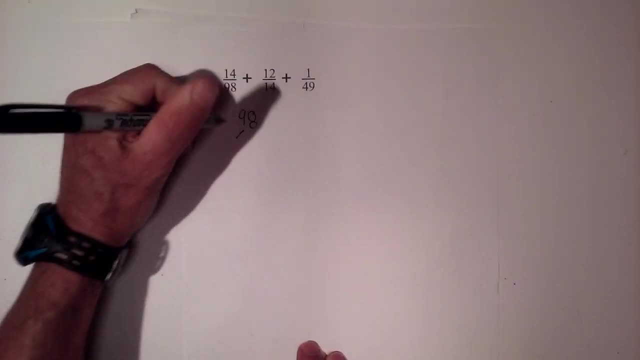 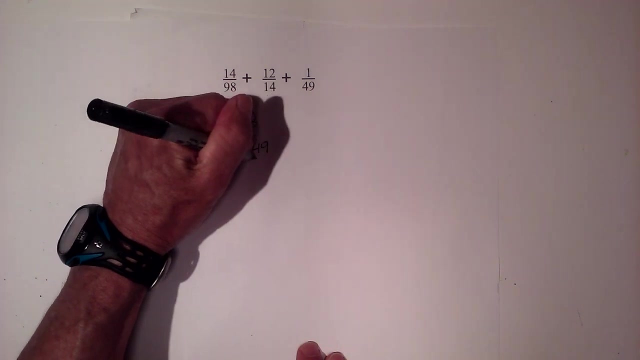 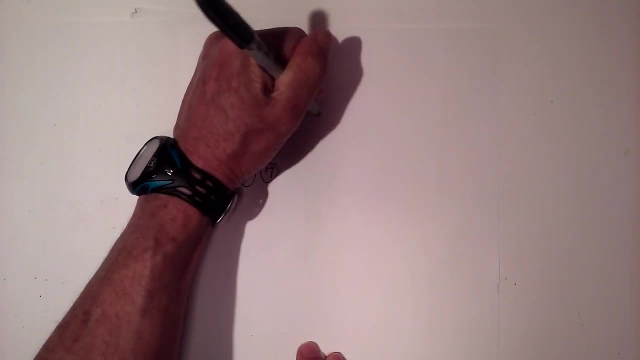 going to do the very same thing. okay, 2 times 49 equals 98.. circle the 2, because it is prime now 7 times 7 equals 49. circle both 7s, because they are prime, now 14. it's a little bit easier, but we have 2 times 7, circle both of these. 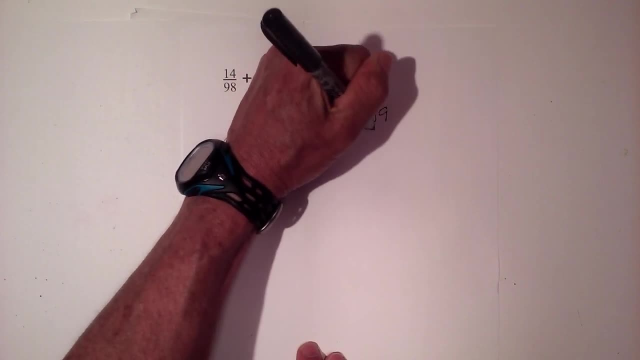 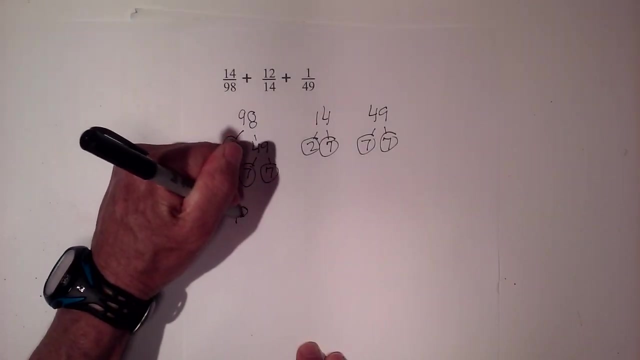 because they are prime and now 49 is just 7 times 7. circle the primes again. i'm going to go back and write down all the prime numbers just to avoid errors. we have 2 times 7 and 7 and then with 14. 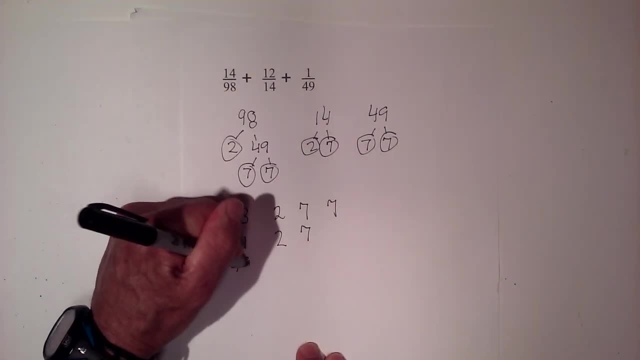 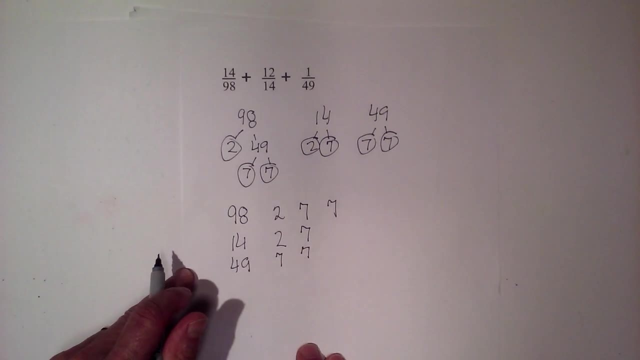 we have 2 and 7, and then, with 49, we have 7 and 7.. okay, let's go through and multiply all these together and apply our one rule. 2 is discovered in two of these, so i'm going to write a 2.